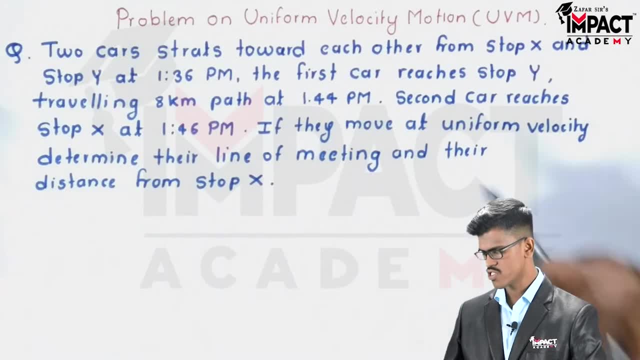 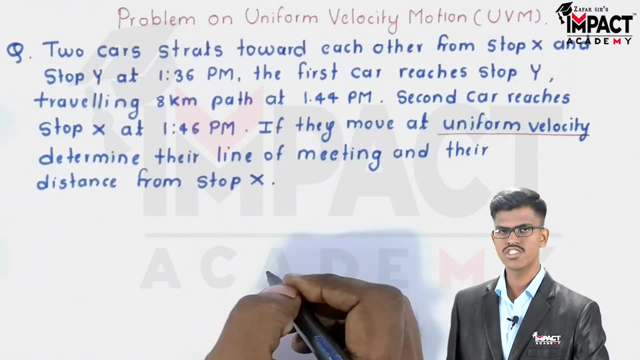 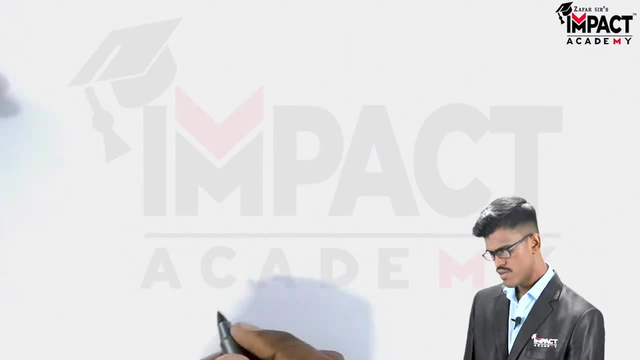 Here. in question they mention a uniform velocity motion. In question they mention a uniform velocity motion. So this is a uniform velocity motion problem. So let's start the problem. In the question they mention two cars. Let's draw a diagram. 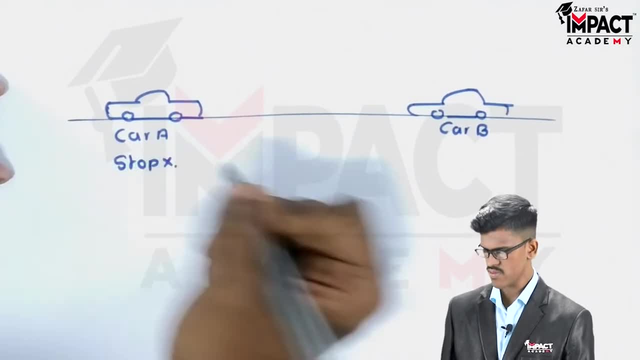 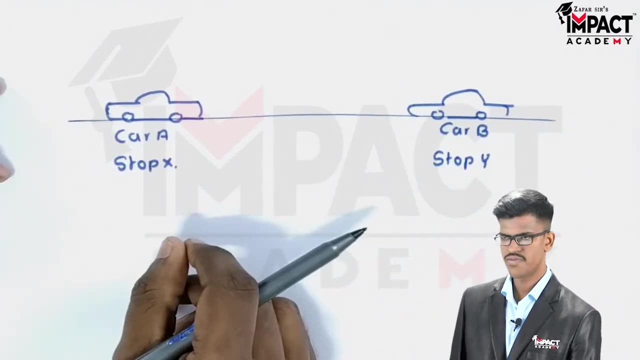 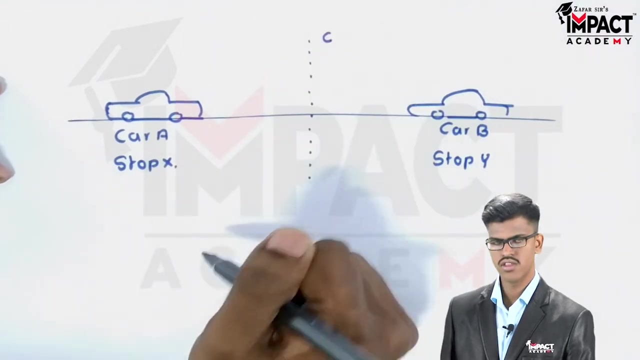 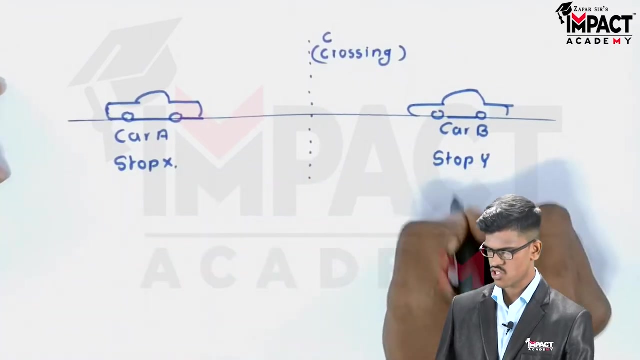 Car is at stop x and car is at stop y. Both the cars started towards each other and meeting at a point- Let's consider point c- in between them, where they cross each other. The distance between stop x and stop y is 8 km, which is mentioned in the question. 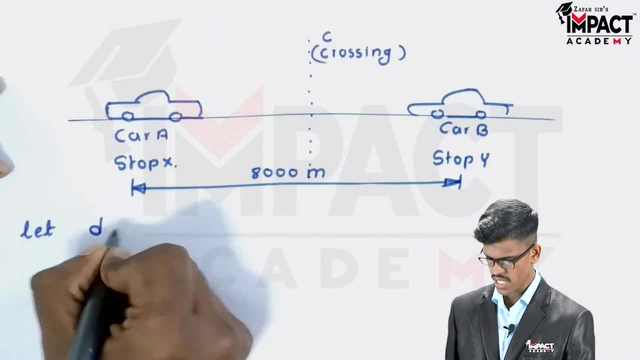 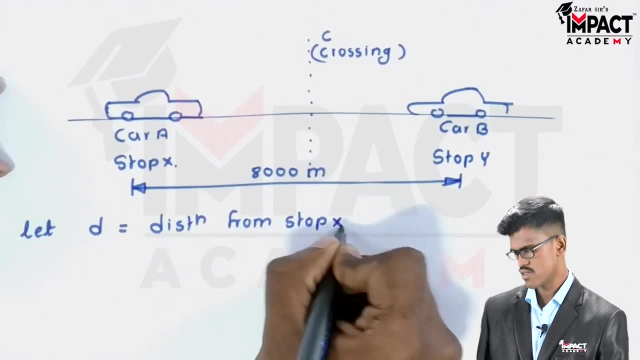 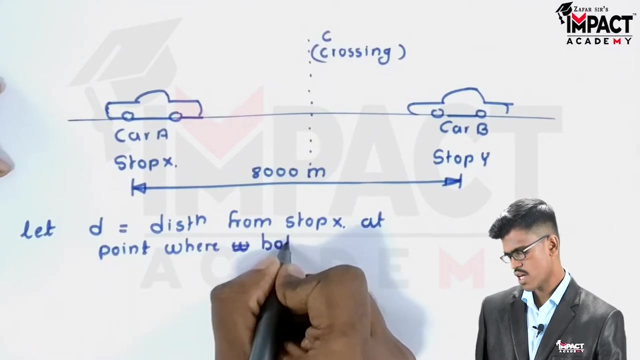 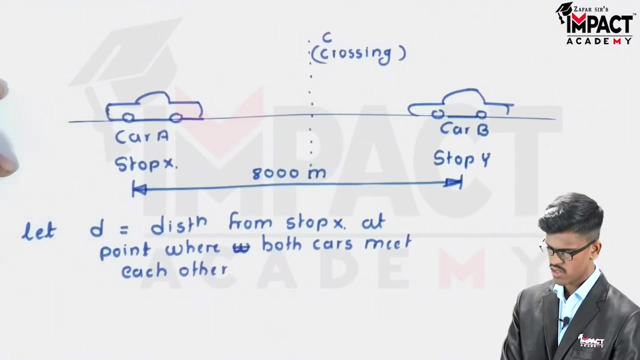 So let's consider D be the distance from stop x at the point where both car meet each other. The distance between stop x and stop y is 1 mind. So let's compare point d with distance from stop x at the point where both car meet each other. 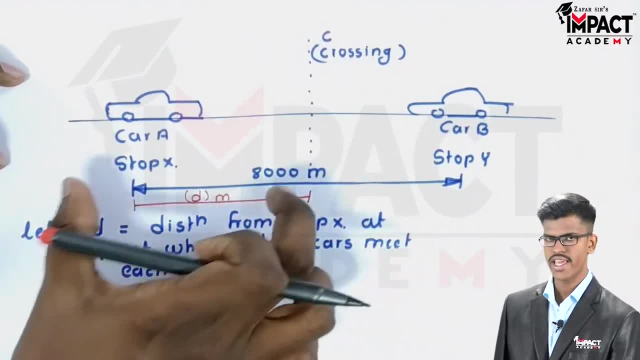 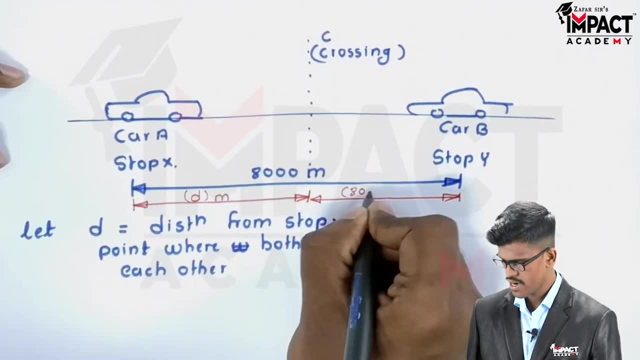 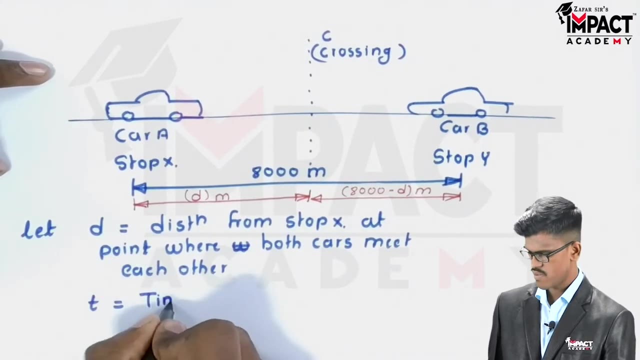 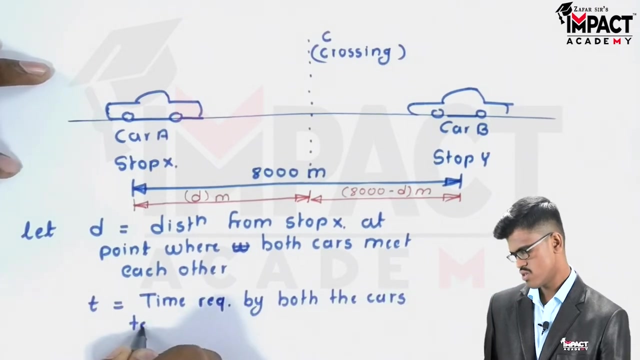 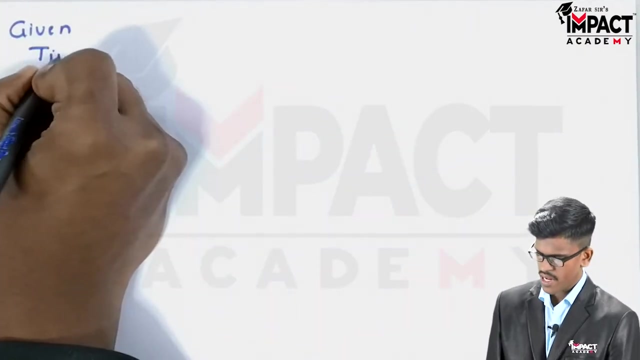 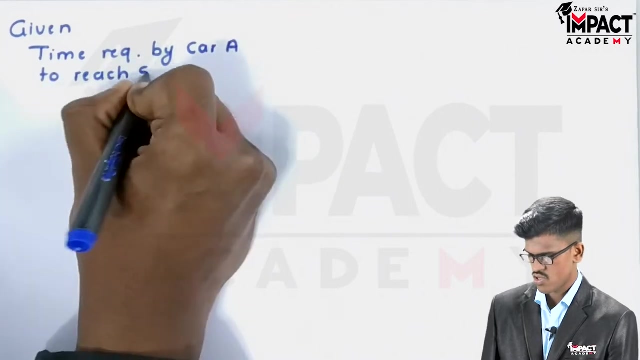 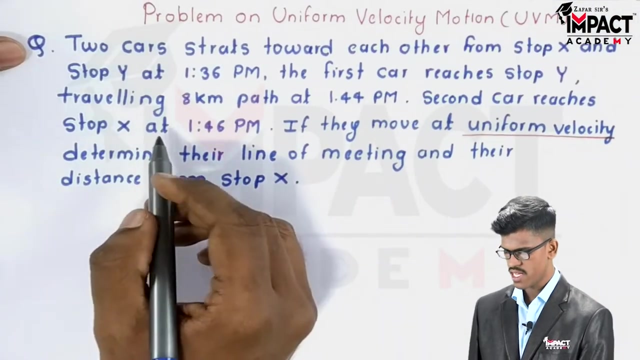 If d is the distance between point x and c, then remaining distance will be 800 minus d, And t be the time required by both the cars to reach at point C. So, given time required by car A to reach stop Y In the question they mention, car A reaches the stop Y Car. 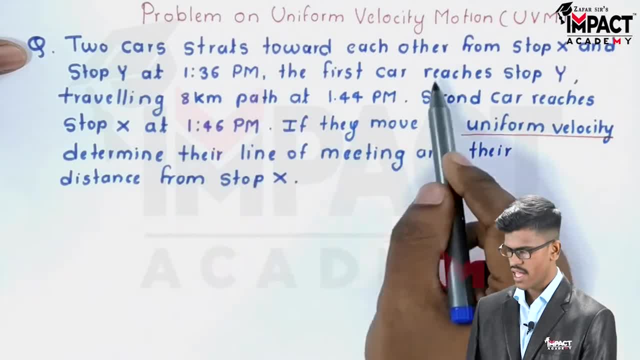 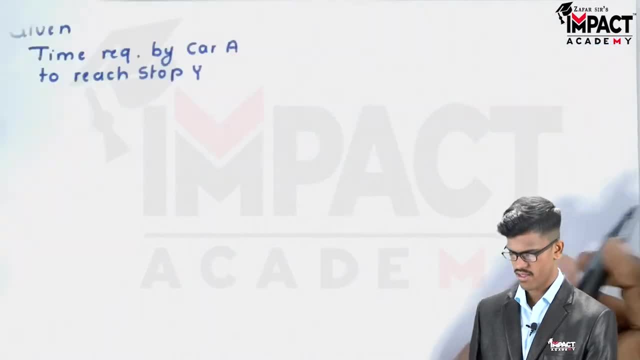 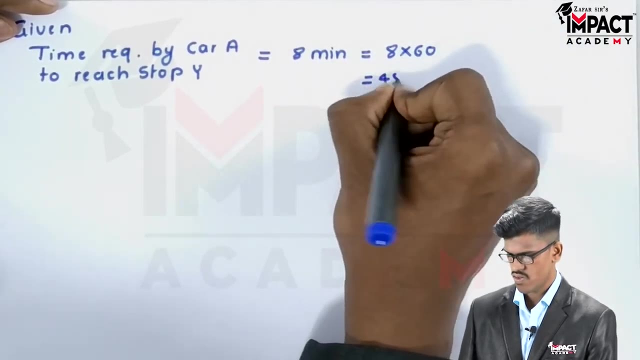 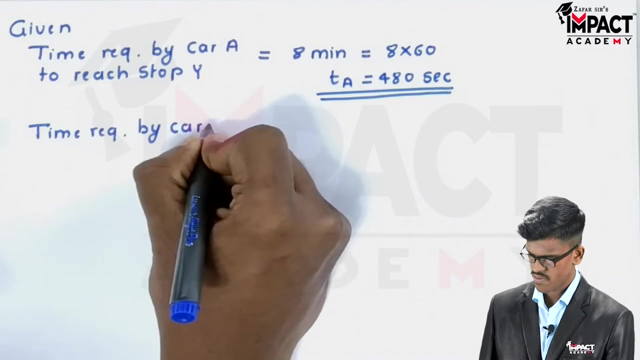 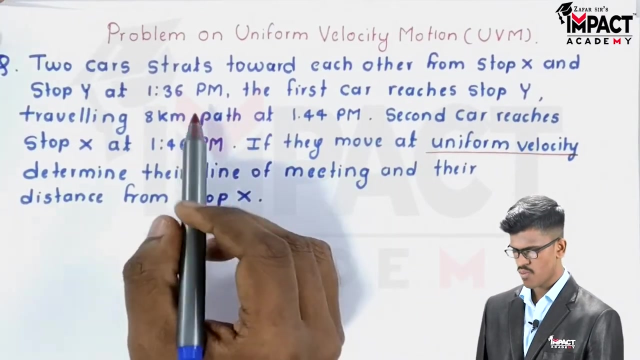 A starts the motion at 1.36 pm and reaches the stop Y at 1.45 pm Means it requires 8 minutes to reach the stop Y. So In the question they mention both the cars. start the motion at 1.36 pm Means car B also. 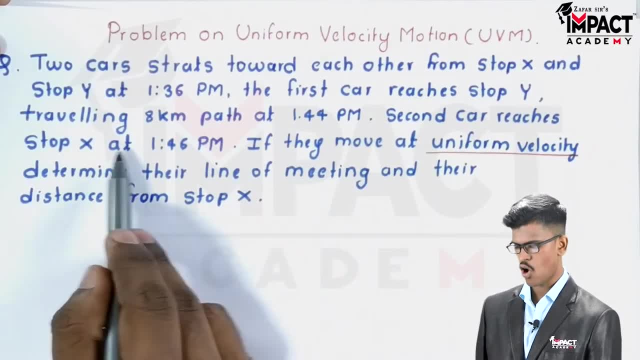 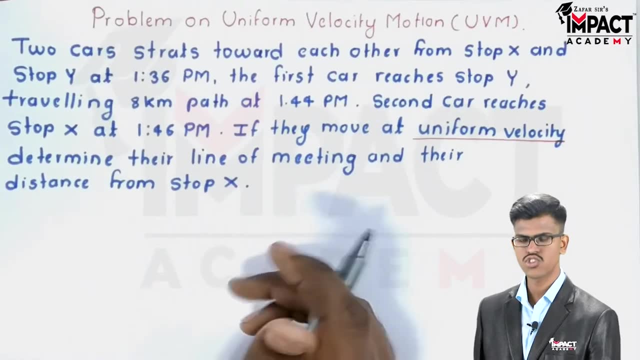 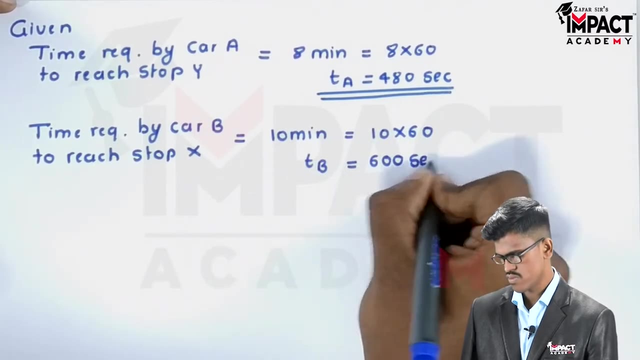 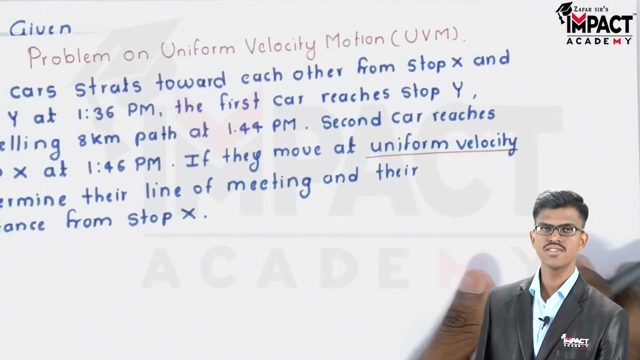 starts the motion at 1.36 pm and reaches the stop X at 1.46 pm. Means Car B requires 10 minutes to reach the stop X. In the question they mention the motion is uniform velocity motion Means there is no. 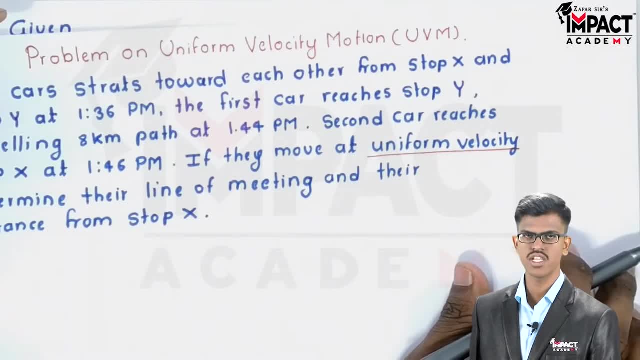 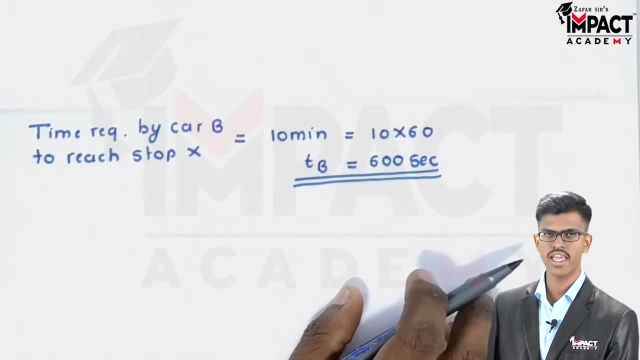 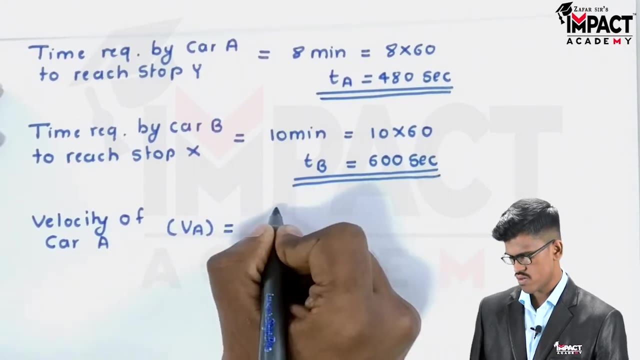 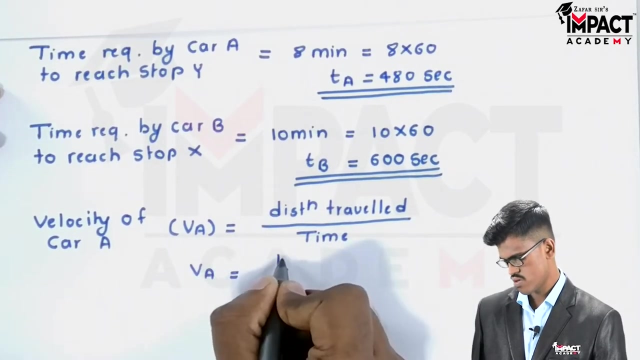 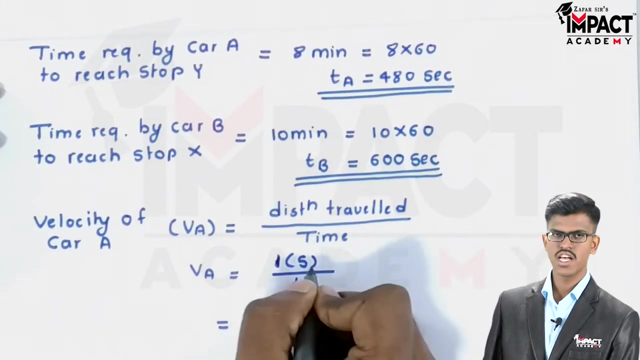 change rate of change of velocity in this motion. Velocity remains constant throughout the motion, So let's find out the velocity of car A and car B Here. Total distance traveled by car a from the from stop x to the stop y is 808 km and time required. 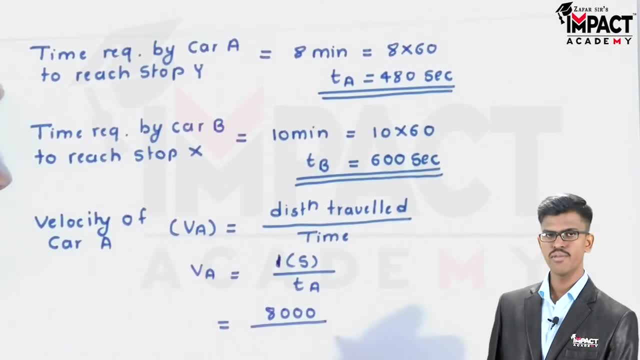 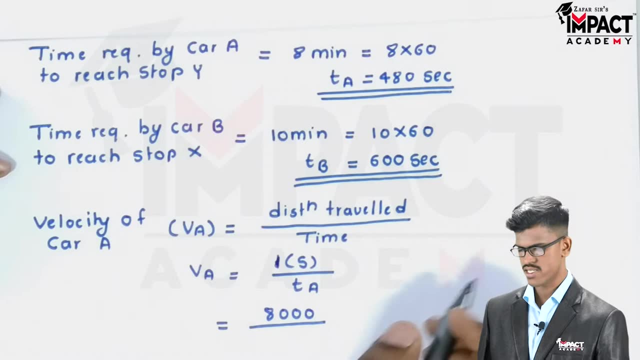 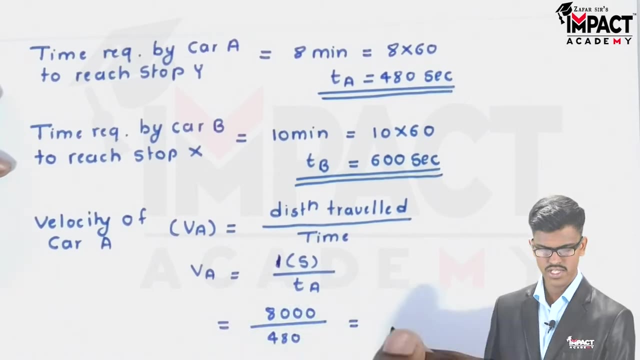 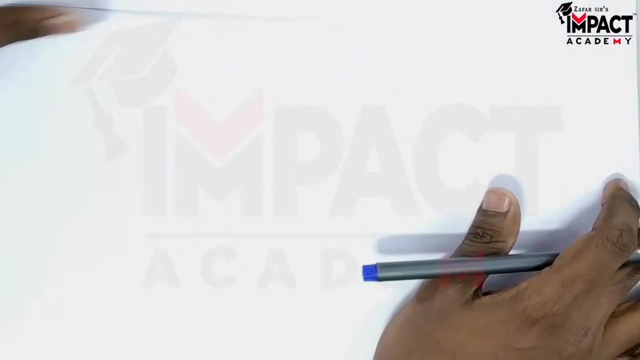 by the car is 840.. What is its distance? required by the car A to reach from stop X to stop Y is 8 minutes 480 seconds. so we get the velocity of car A, which is. this is the velocity of car A. let's find out the velocity of car B. 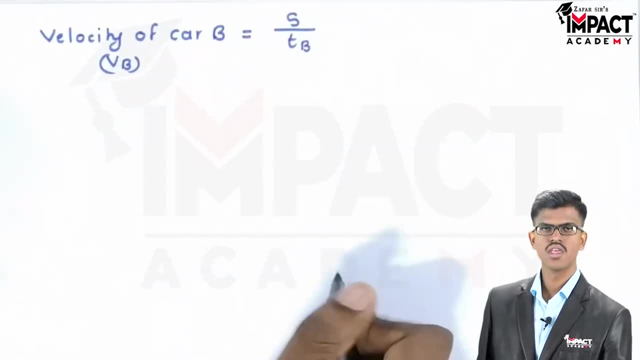 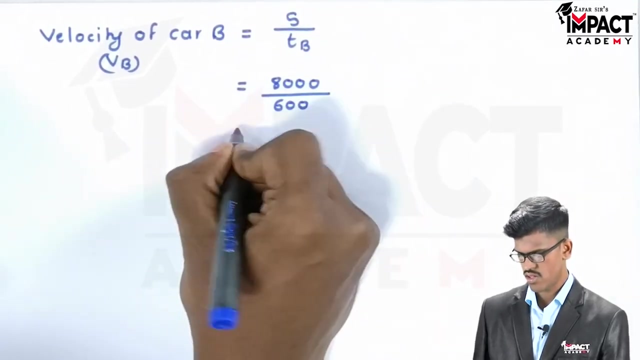 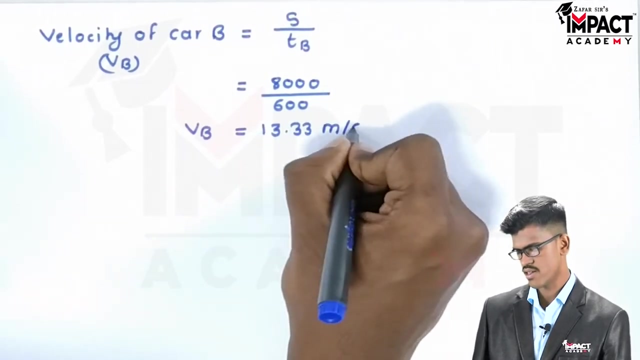 here a car B travel a distance from point X, point from point Y to point X, which is 8 kilometer and required times 10 minutes. so velocity of car B will be 13.33 meter per second. okay, now we have to find the inequality of the velocity of car B. 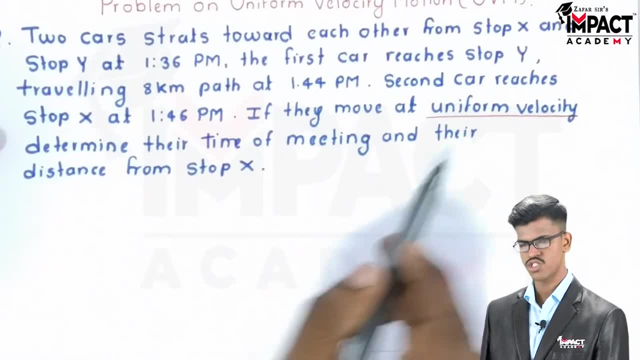 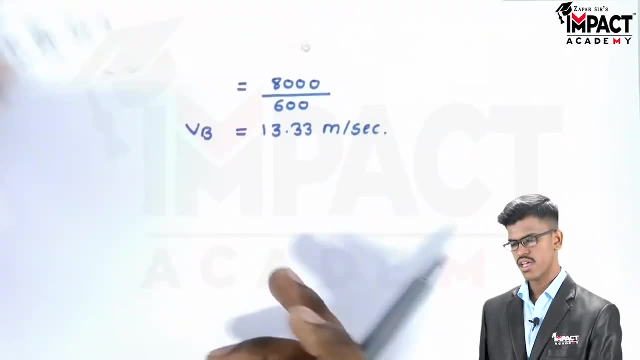 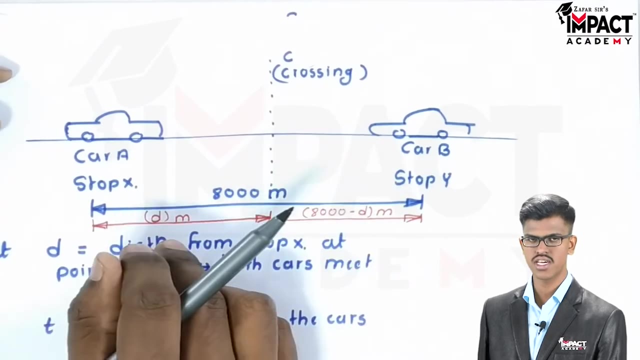 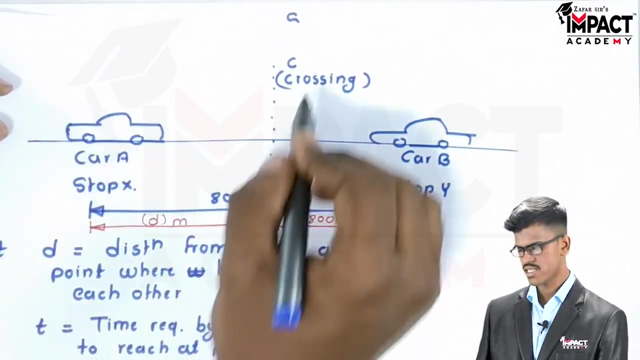 in the question dimension, it is a uniform velocity, dimension, motion, and we have to find the time of meeting and their distance from X. in diagram we mention a point C where car A and car B just cross each other and they meet each other at a point C. so we have to find the distance D from stop X up to point C where they 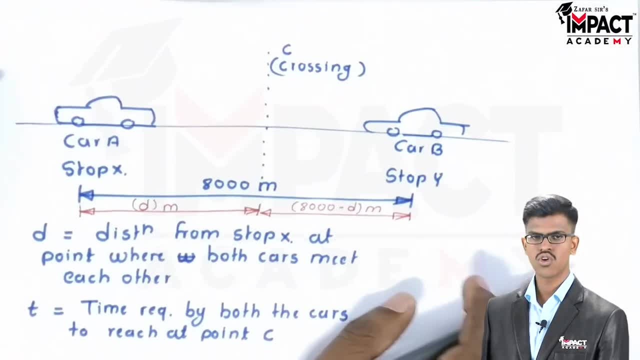 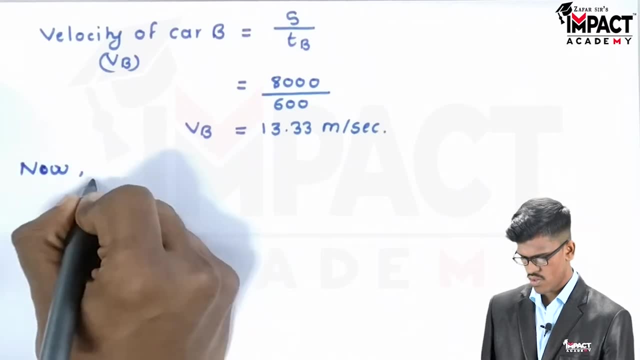 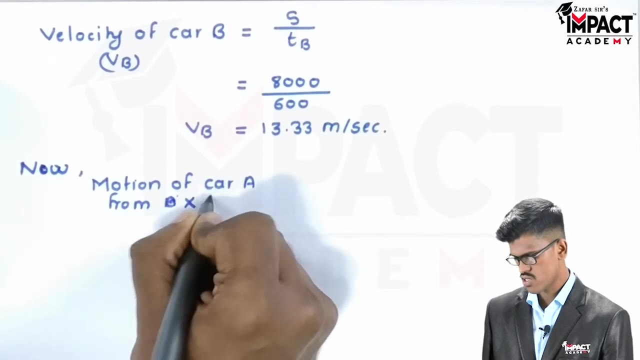 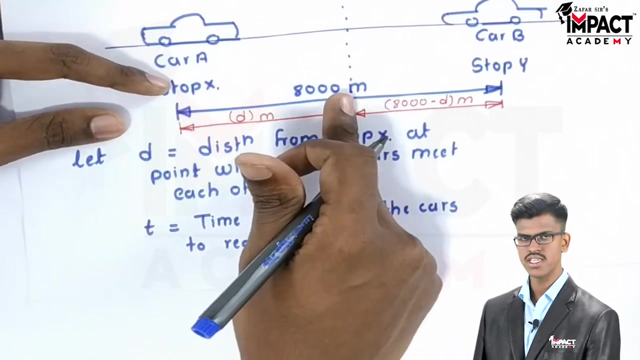 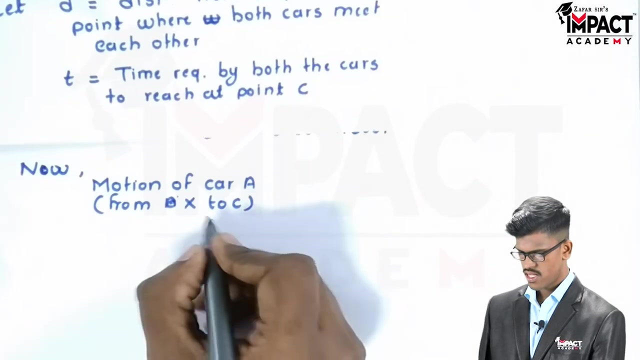 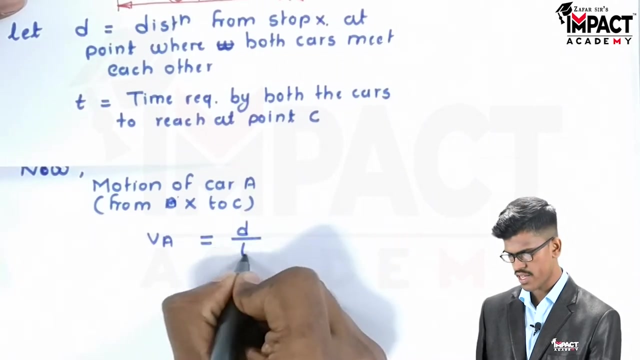 cross each other and I am required to cross the point C. now, motion of car A from X to C, from point X to point C. car A travel distance D and required time is T, and then velocity of car a becomes VA is equal to be D upon t. we know the. 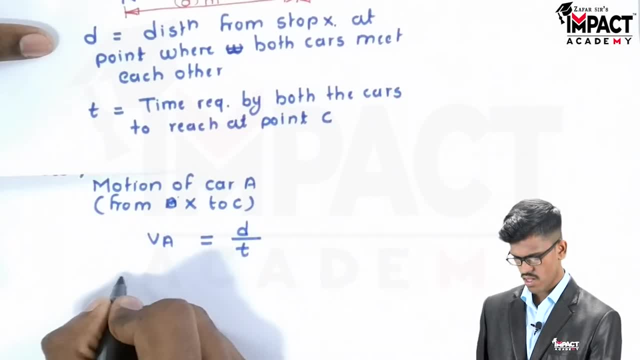 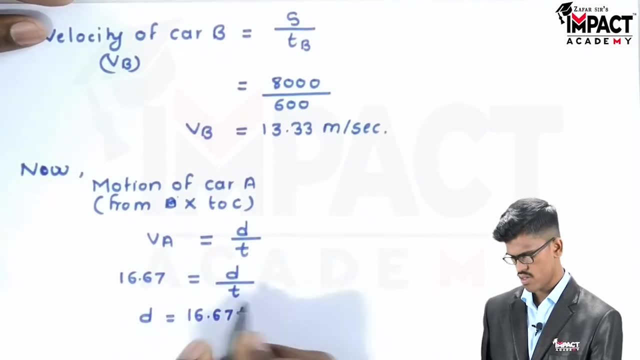 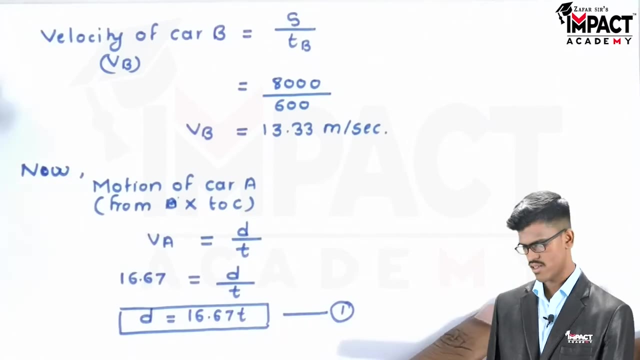 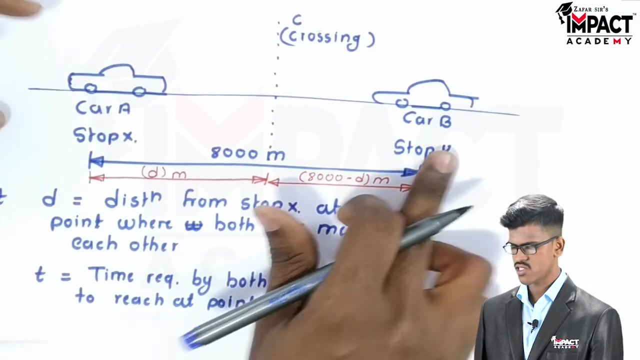 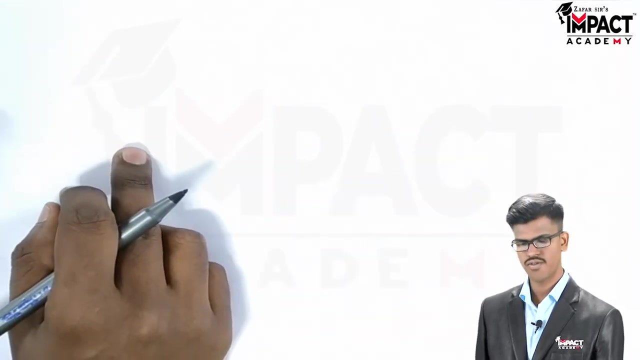 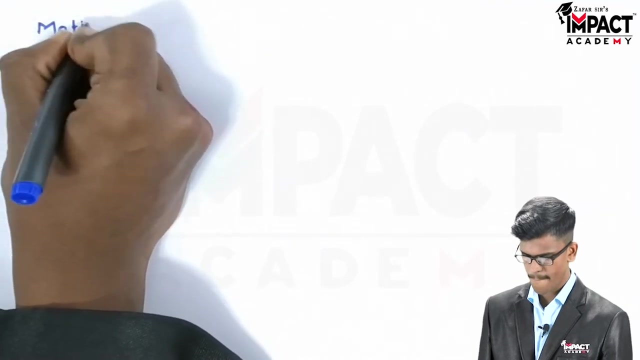 velocity of car A, which is 16.67. so we get a first equation: D is equal to 16.67. Now consider motion of car B from stop X to stop C, from point C. Now we consider motion of car B from stop Y to point C. 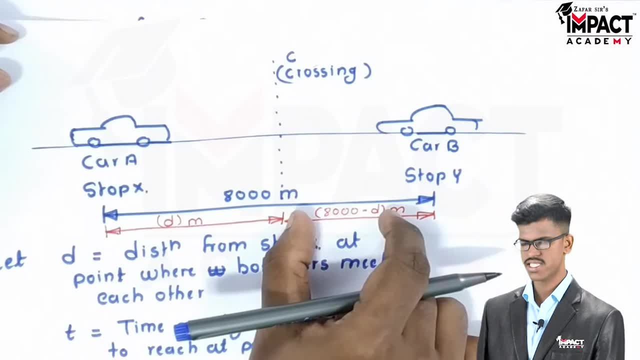 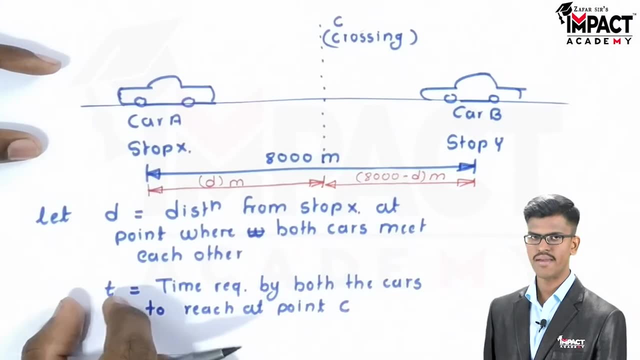 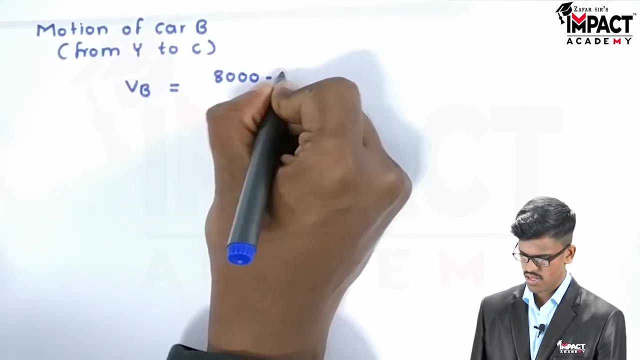 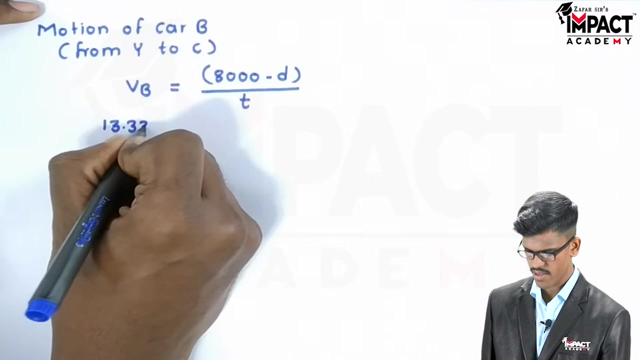 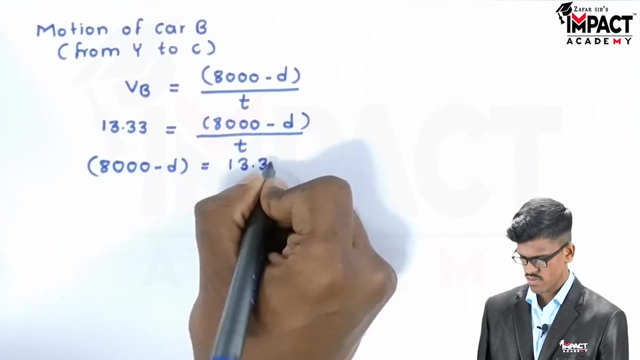 From point Y to C. car B travel distance 800-D meters and required time for the car B is the same time, T. Then the velocity of car B becomes the same. We know the velocity of car B, which is 13.33.. 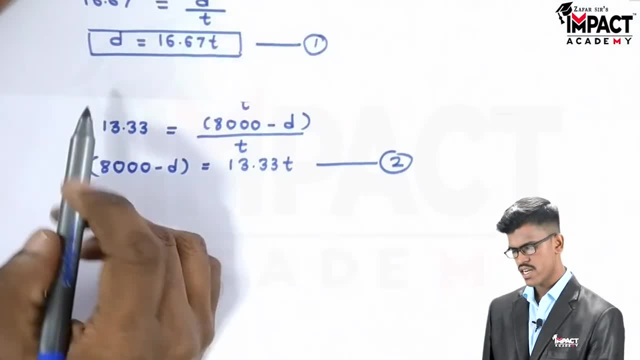 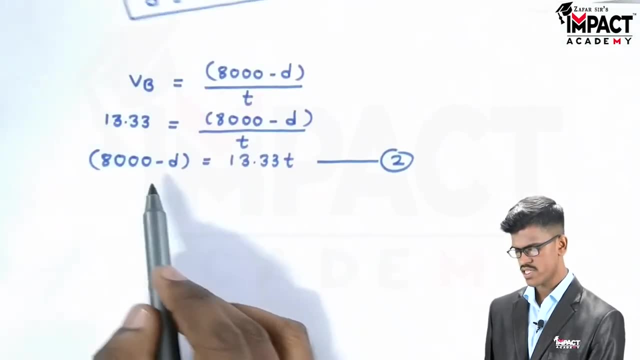 So we get two equations. Equation number 1 is D is equal to 16.667 T. An equation number 2 is D is equal to 16.667 T. An equation number 3 is D is equal to 16.667 T.